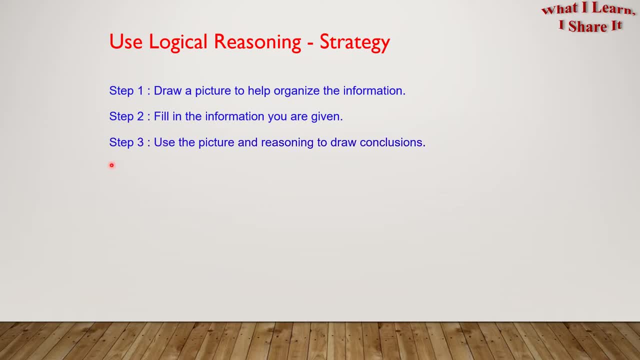 Step 3. Use the picture and reasoning to draw conclusions. Here's the problem. to help us understand the strategy, What is the date of Ellie's birthday in July? Use these clues to decide. The date has two digits. The sum of the digits is 8.. 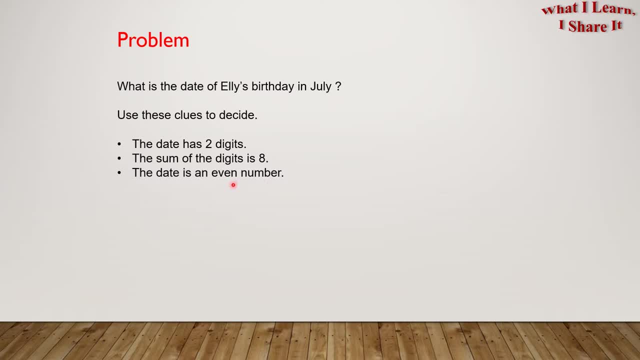 The date is an even number. Do you want to try it yourself? Feel free to pause the video and try it yourself. Do you want to see how I solved it? I solved it in a step-by-step way. Let's see it. 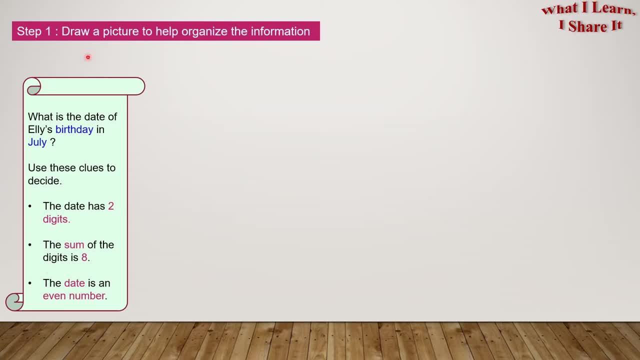 Step 1. Draw a picture to help organize the information. So what information do we have? We have the information that that Ellie- Ellie's birthday is in July. So we are going to draw the dates in July And here it is. 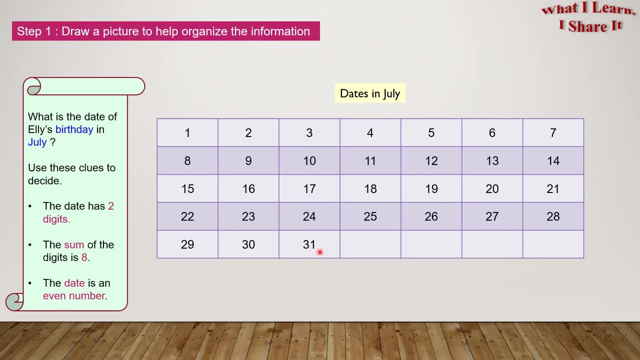 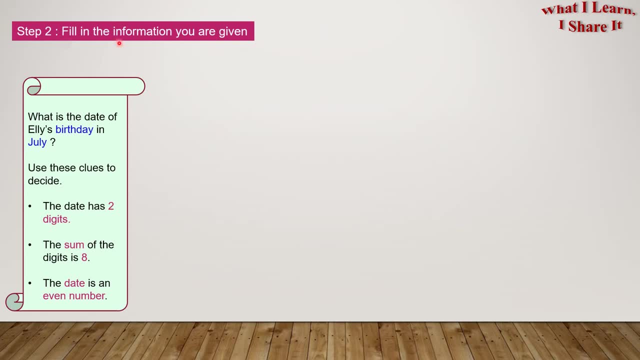 The 1st of July to the 31st of July. Step 2. Fill in the information you are given. So what is the information? We are given the information as clues in here. We are given the information as clues in here. 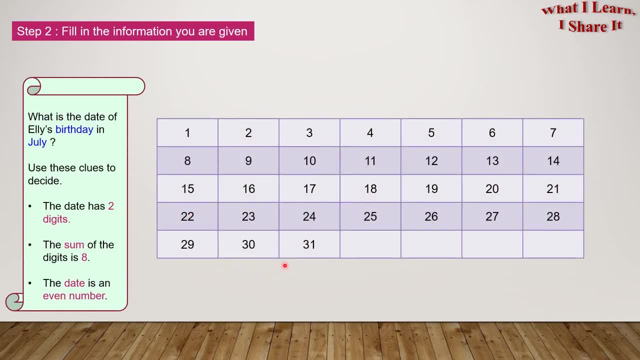 We are given the information as clues in here, And here's our table again, Clue 1. The date has two digits. Nope 1 doesn't have it, So we are going to cross out each of the one-digit numbers. 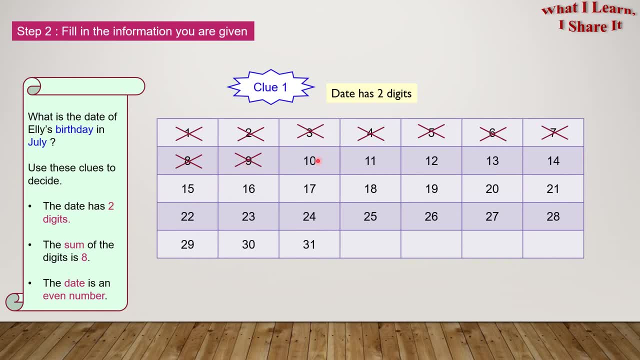 And numbers 1 through 9 are crossed out. So numbers 10 to 31 are remaining. So numbers 10 to 31 are remaining Clue 2.. The sum of the digits is 8.. 1 plus 0 is 1.. 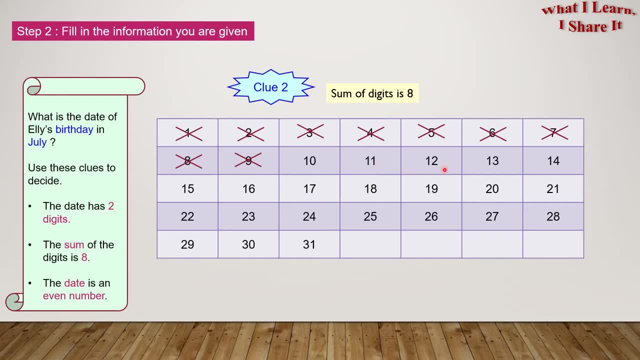 1 plus 1 is 2.. Let's see: Aha, 1 plus 7 is 8.. 1 plus 8 is 9.. 22 plus 6 is 9.. Aha, 2 plus 6 is 8..